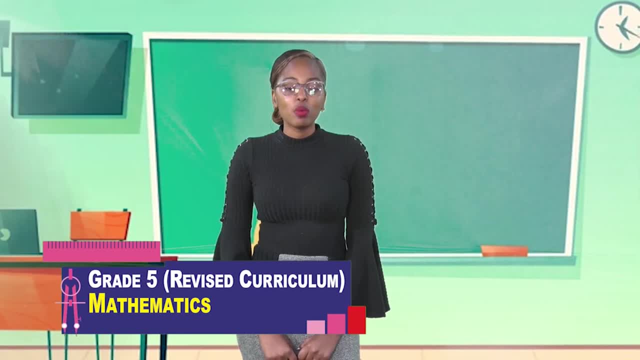 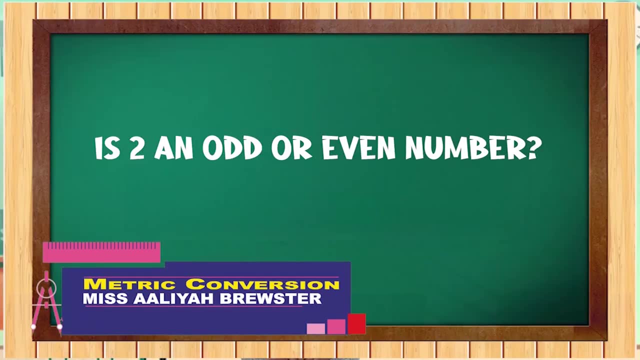 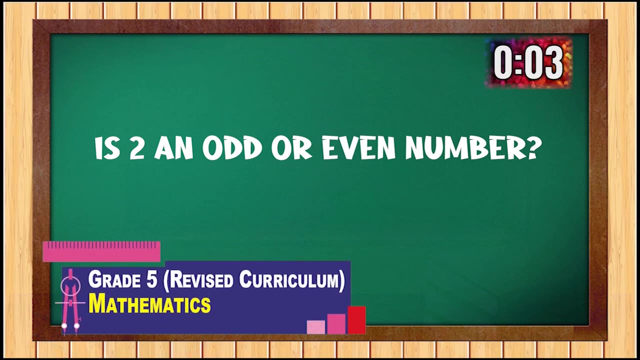 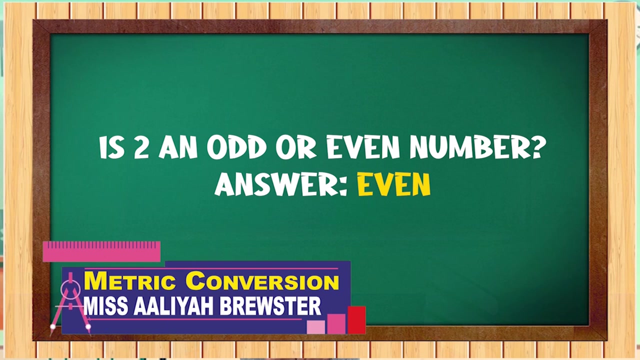 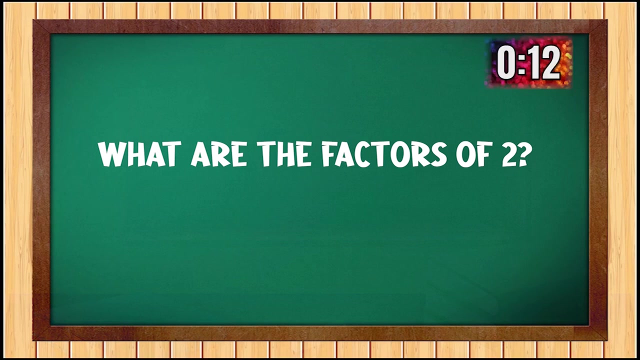 Our second warm-up activity is we'll be looking at questions revolving around the numeral two. First question: is numeral two a odd or even number? It is a even number. What are the factors of two? The factors of two are one and two. 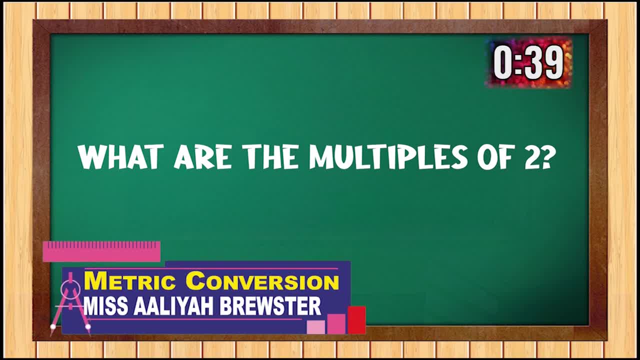 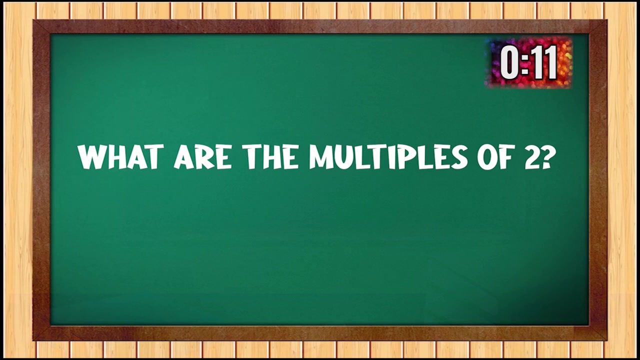 What are the multiples of two? What are the multiples of two? What is one? We'll discuss minutes and seconds, then your assumptions. Who's Hottie? We'll talk about who's Hottie and what they're really like. Your assumptions are from what you do. 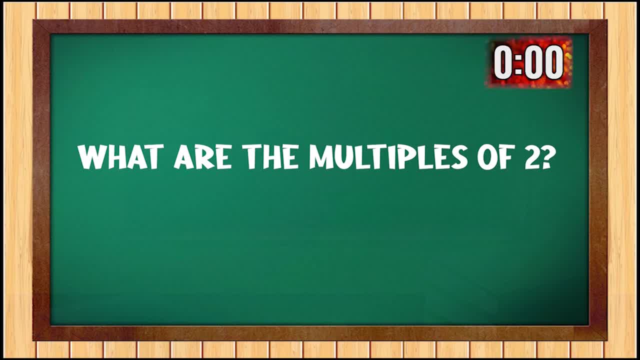 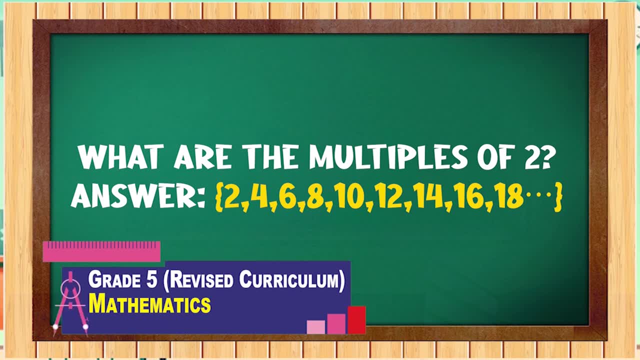 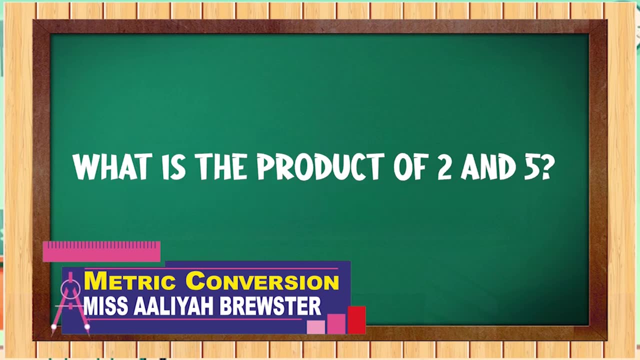 well, The multiples of 2 are 2,, 4,, 6,, 8,, 10,, 12,, 14,, 16,, 18, and we can go on. What is the product of 2 and 5?? 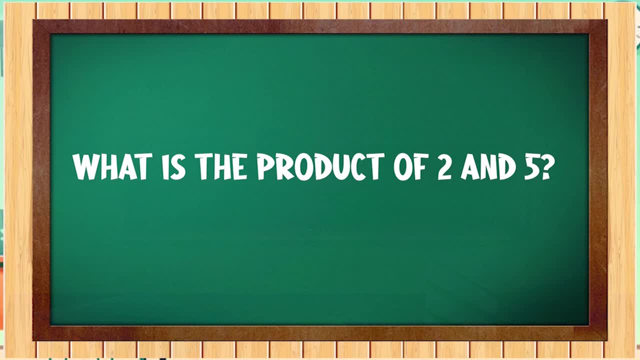 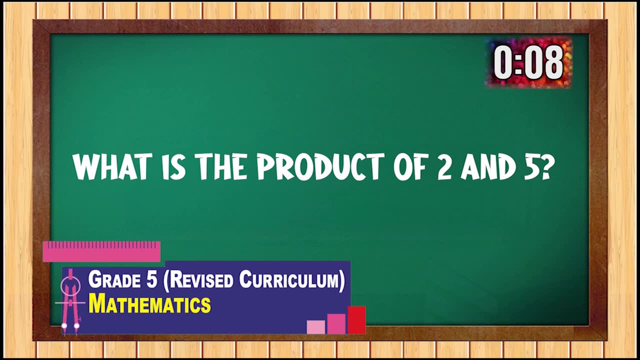 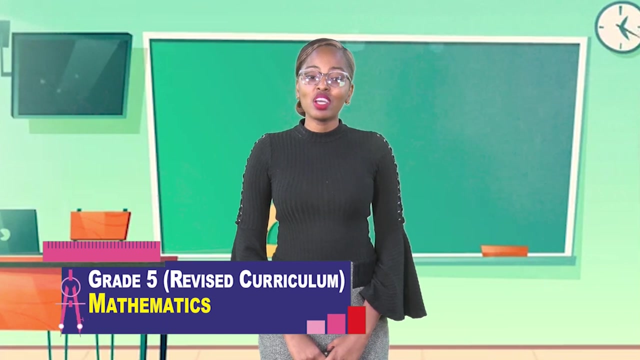 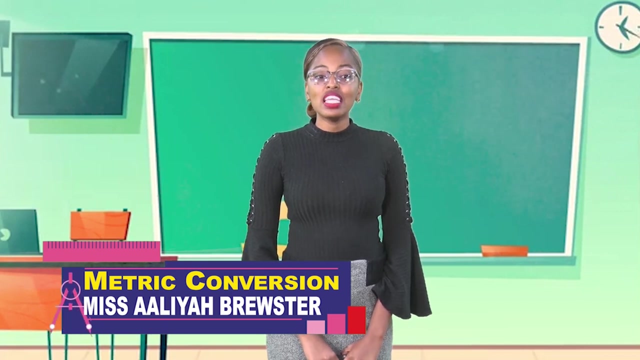 In this instance, product means multiplication. So what is the product of 2 and 5?? The product of 2 and 5 would be 10.. Before we begin our lesson- that is, measurement- we'll start off with a story. The name of this story is: How Big is a Foot? 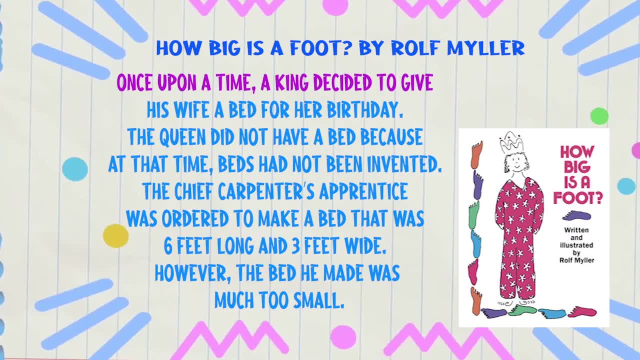 By Ron Rolf Miller. Once upon a time a king decided to give his wife a bed for her birthday. The queen did not have a bed because at that time beds had not been invented. The chief carpenter's apprentice was ordered to make a bed that was six feet long and three 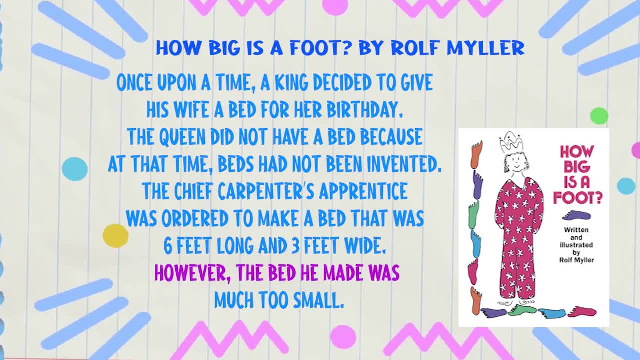 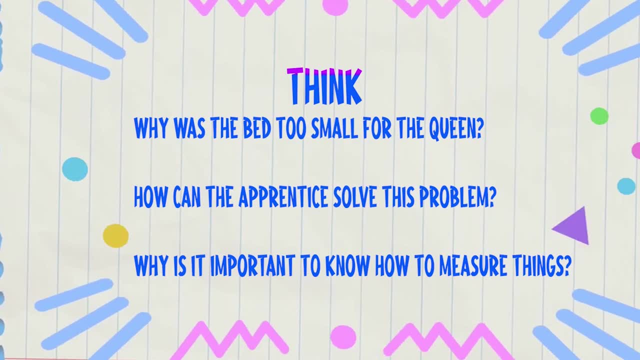 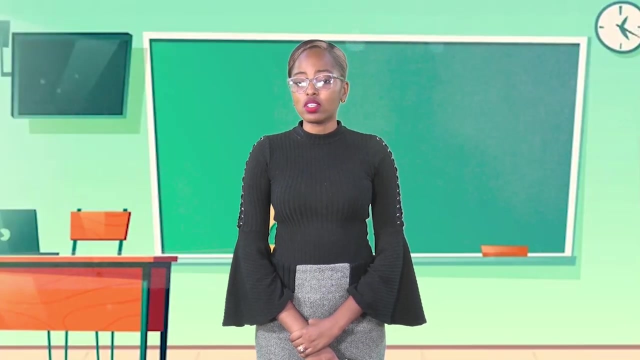 feet wide. However, the bed he made was much too small. Think for a while. Why was the bed too small for the queen? How can the apprentice solve this problem and why is it important to know how to measure things? Measurement is very important to us. 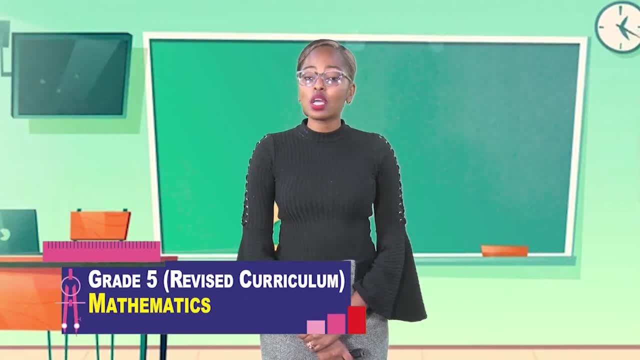 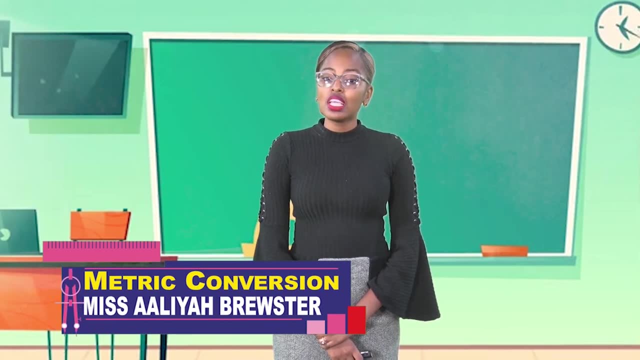 When Mommy is baking a cake, she has to know the exact amount of ingredients to use for that cake to be perfect. The carpenters or builder has to be certain that the blocks are wood and the material at the heaps be flat. So you can cool your money. 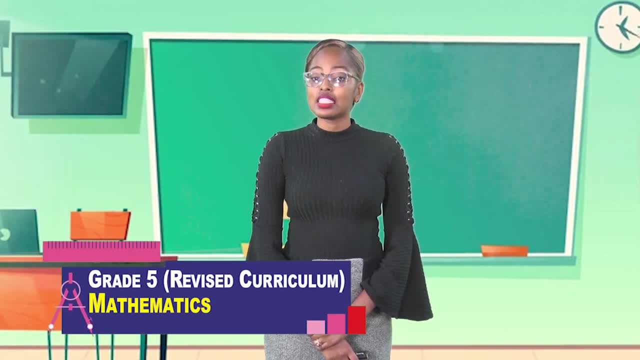 Her husband does the work and my agricultural business. Masterful at work, My husband can teach you to soybeans and job design And he doesn't spend so much time in worldça fishing that sometimes he doesn't get the work done. has the precise shape so that it can rest in the exact space to make a house. 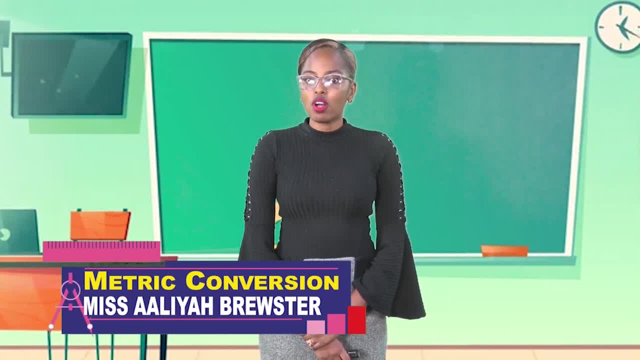 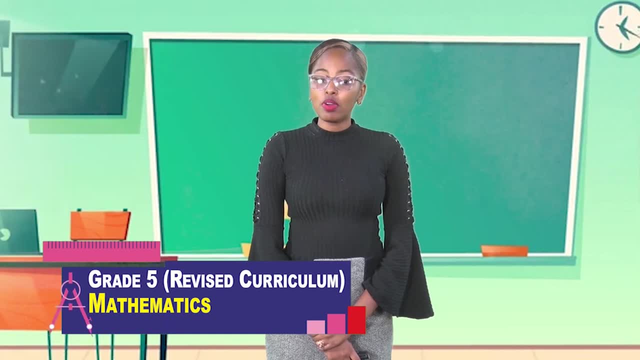 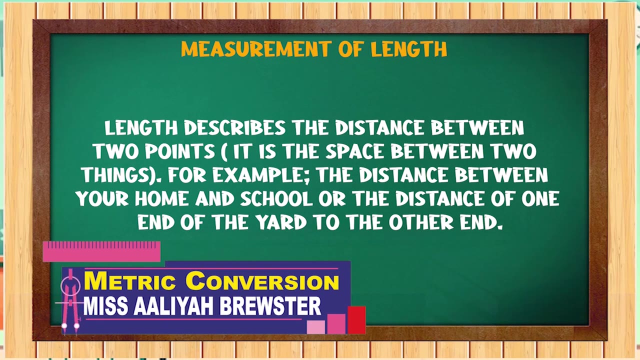 If he or she cannot measure properly, the house will fall apart. In the story we realize the bed was too small for the queen because the apprentice did not understand measurements. Let's continue with the measurement of length. Length describes the distance between two points. 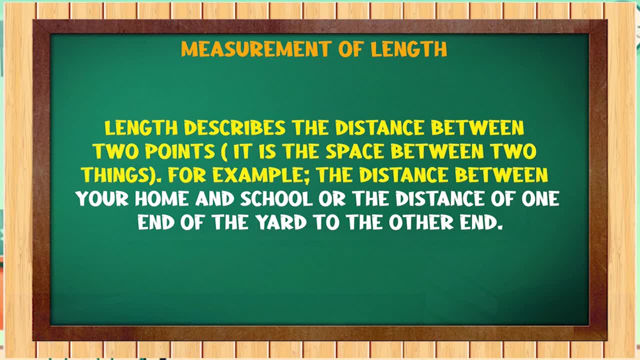 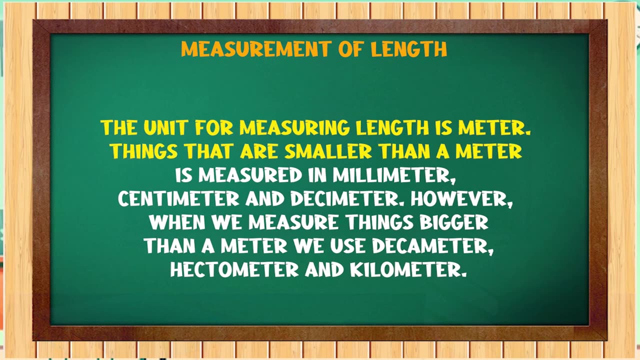 That is the space between two things, For example the distance between your home and school, or the distance from one end of the yard to the other end. The unit for measuring length is meter. Things that are smaller than a meter is measured in millimeters, centimeter and decimeter. 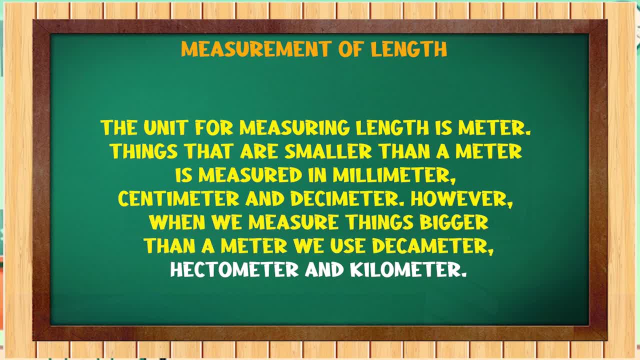 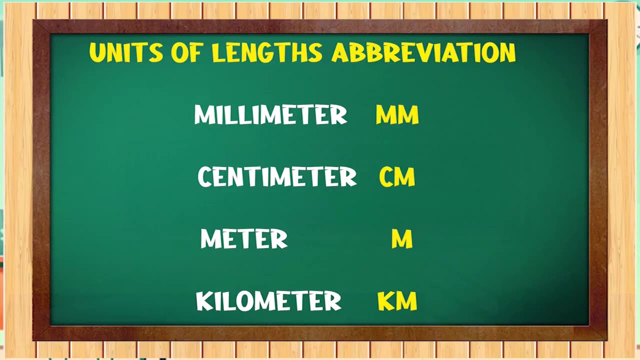 However, to measure things bigger than a meter, we use decameter, hectometer and kilometer. Let's now look at the abbreviation for these units of length: Millimeter is represented by mm, centimeter is represented by cm and meter is represented by m. 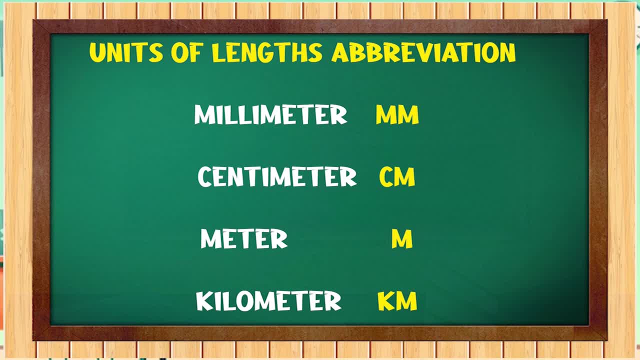 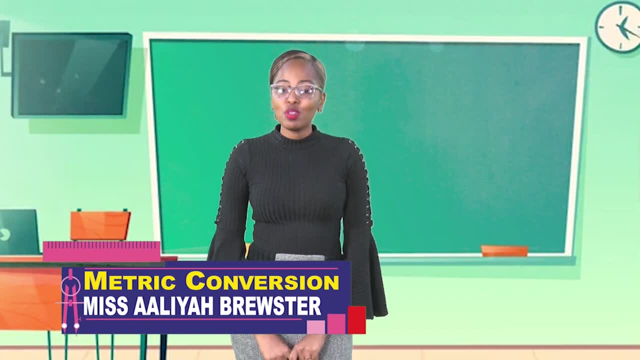 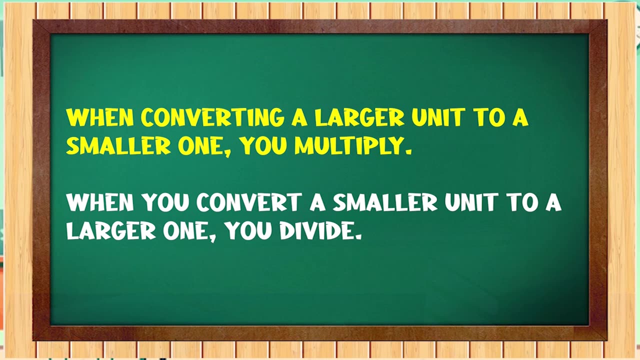 while kilometer is represented by km. Now we'll move on to converting units of length. This concept is simple if you understand it in this manner. If you are converting a large unit to a small unit, you have to multiply. However, if you're converting a small unit to a large unit, you divide. 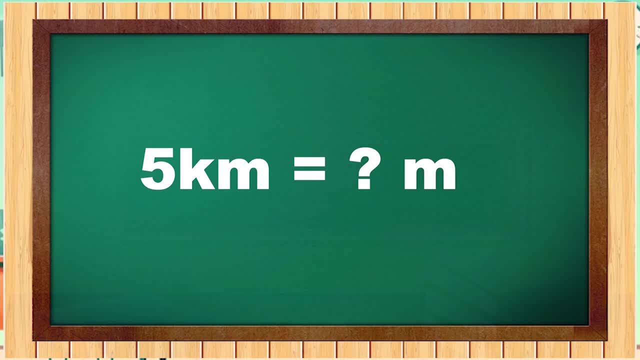 Examples: if you're asked to convert five kilometer to meter, you have to multiply Because kilometer is large. you have to multiply Because kilometer is large. you have to multiply Because meter is larger than meter. Hence, we're being asked to change something that's large into something that's small. 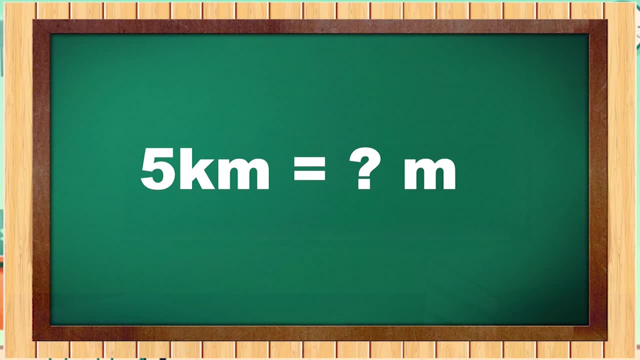 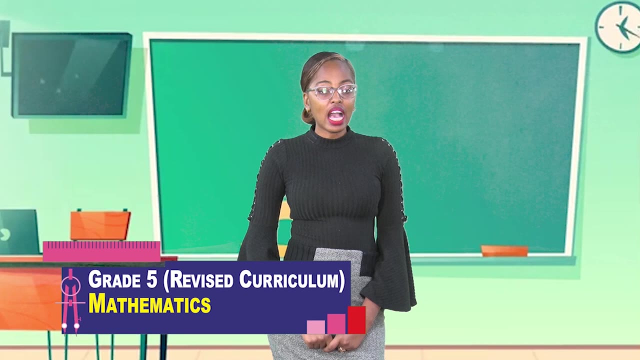 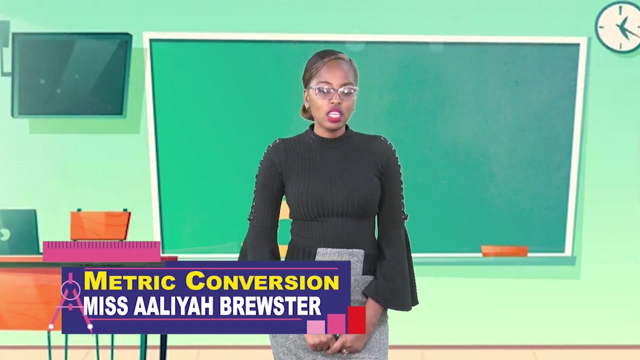 Therefore we must multiply. So the working would be to multiply five times one thousand and the answer would be five thousand meter. However, there are times you may be asked to convert a small unit of length to a larger unit of length. in those instances we divide, for example, 1500. 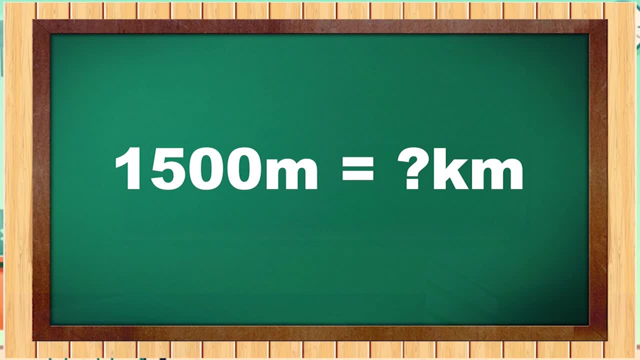 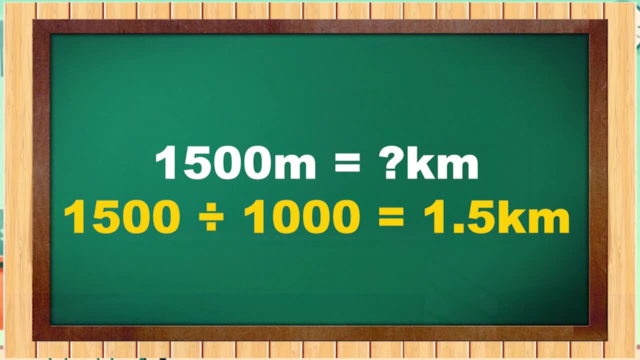 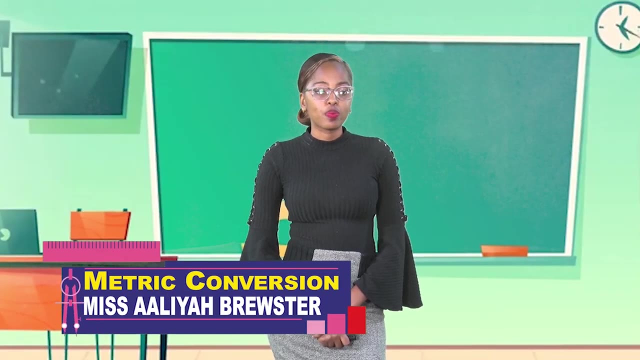 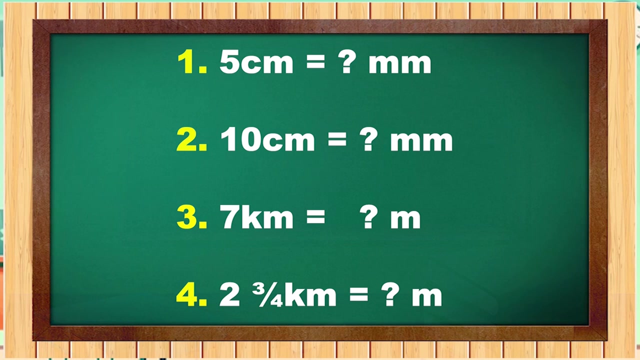 meter converted into kilometer means that we must divide 1500 by 1000, and that would give us 1.5 kilometers. now you can try this activity on your own. number one: convert 5 centimeter to millimeters. number two: convert 10.